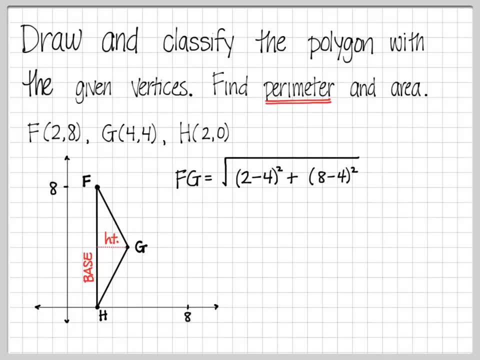 Subtract your X's and square it. Add that to the difference. so subtract your Y's and square that And we get negative 2 squared plus 4, squared which is 4 plus 16, which is the square root of 20, which reduces to 2 root 5.. 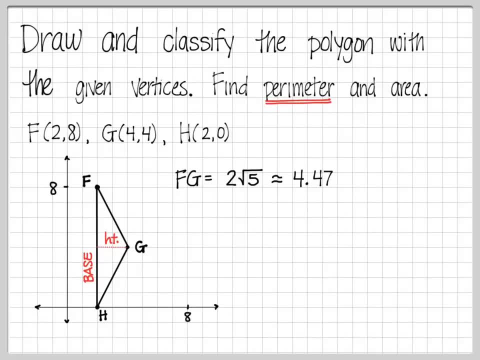 And we're going to also write the decimal approximation for that. We want both of the exact and the approximate for each one of these, And what we're hoping for is that when we look at the measure of G H, we're going to get the exact same thing. 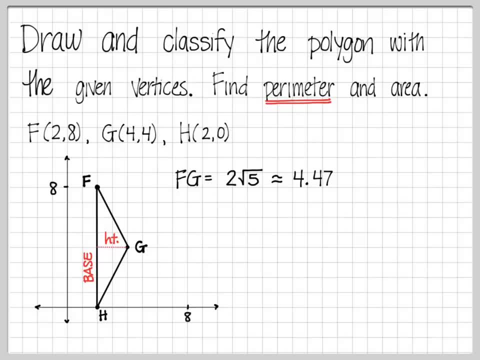 Because we saw that by critically reasoning this, we could see that they are the same length. So I take the difference of my X's and the difference of my Y's, square each of those differences and add it together And I get 2 squared plus 4 squared, which is 4 plus 16.. 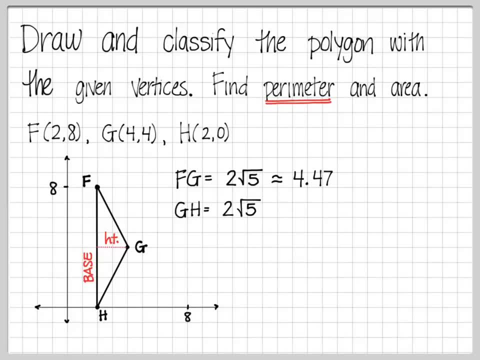 Square root of 20, which is exactly the same thing as FG. the length of F to G, which is 2 root 5.. And again the decimal approximation. So our critical reasoning was correct in the beginning and our algebraic, our computational distance formula showed that we were correct. 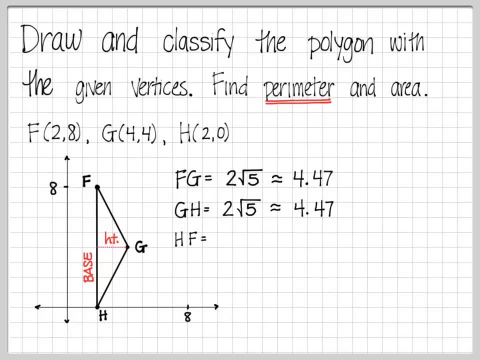 Now to find the distance from H to F. I could use the formula again, But we said in the very beginning: we noticed that from H to F it's a vertical line. We can just count the squares and we see that it's 8 units. 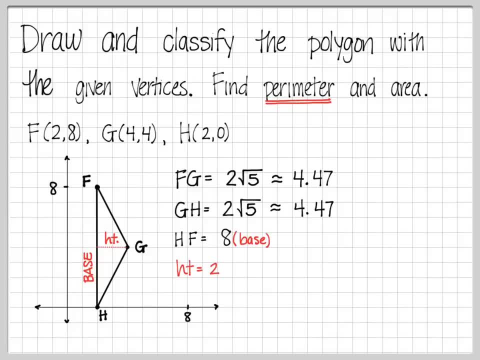 And we call that our base and we can count the squares again to find our height, which is 2.. So we have two ways now to actually prove that we've shown that this is an isosceles triangle. So we're very, very firm in our knowledge that it's an isosceles triangle. 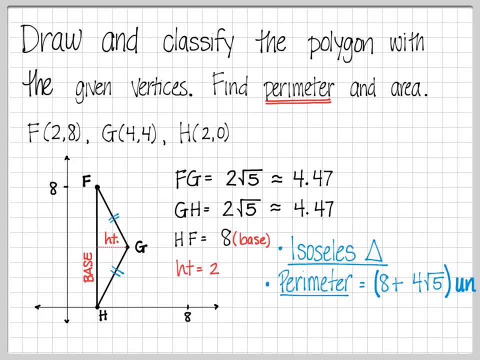 The perimeter. well, we add up each of those lengths: the 2 root 5, the 2 root 5, and the 8. And we get 8 plus 4 root 5 units. That is the exact perimeter. 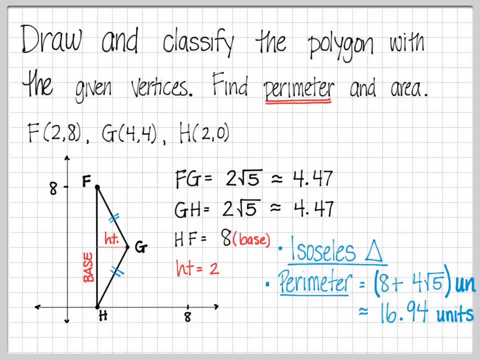 The approximate perimeter would be to add the decimals up, We get 16.94.. To find the area, we do half of the base, times the height, And so that would be 1 half 8 times 2, which is 8 units squared. 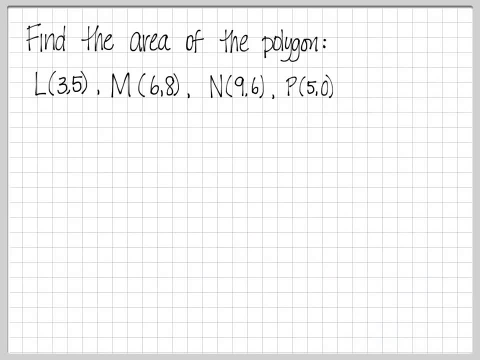 For our second example. this time we have four vertices. So once again we need a coordinate plane And we have it labeled with the scale On the axes. we graph the four points and connect them. And we might first do a little bit of critical reasoning and say: 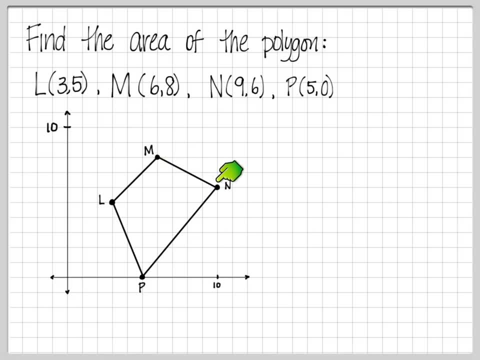 well, I can tell that it's not a parallelogram, because it's very clear that the side MN and the side LP are not parallel. But what about the side LM and the side PN? Well, the rise and the run for LM. the rise, I go up 3 and I run 3.. 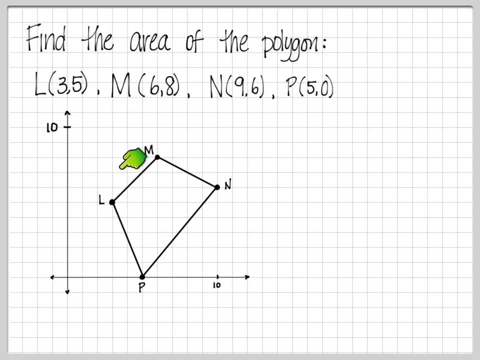 So the slope from L to M rise to run, the ratio is 1 to 1.. So this is a slope of 1. From P to N, I rose 6 and ran 5. It does not have a 1 to 1 ratio. 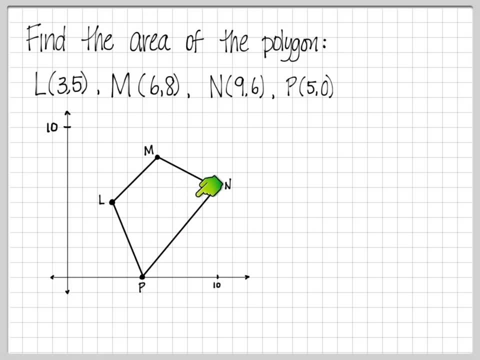 This slope is not 1.. It would be 6 divided by 5.. Okay, that would be that slope. So these two sides are not parallel. There are no parallel sides. Therefore, this is an irregular polygon. It's not a parallelogram or any of the types of parallelograms we know. 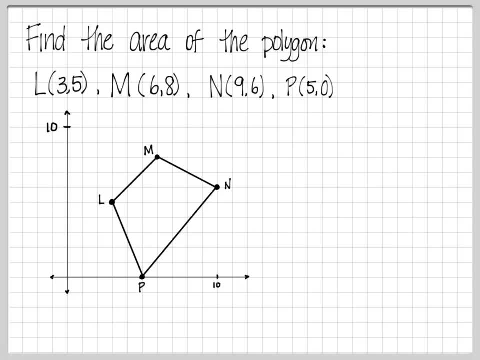 It's not a trapezoid And it's not a kite. So therefore, we have to use how to find the area of our irregular polygon, And the step for that is to have it inscribed within a rectangle, meaning each of the four vertices. it has a point on the sides of a rectangle. 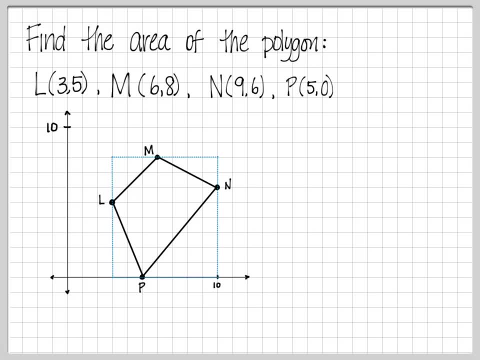 So that blue rectangle has been circumscribed about or inscribed, has the quadrilateral inscribed within it And we can count the squares. It's different. We're going to find the length and the width of that rectangle, so it's 8 by 7.. 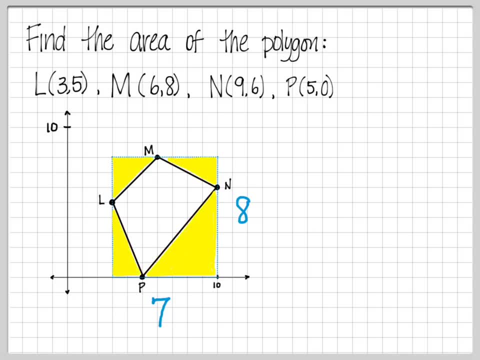 Then we're going to look at the four triangles and we're going to find the area of each of those triangles. Well, this first triangle has dimensions of 3 of the legs, or 3 and 3.. So the area would be 1 half 3 times 3, 1 half of 9, which is 4.5. 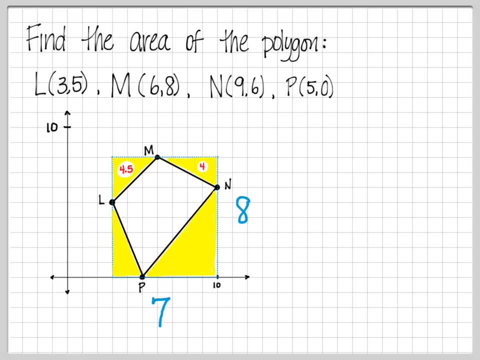 The second triangle would be 1 half 2 times 4, so it's going to be 4.. And this third triangle is 1 half 6 times 5,, which is 1 half of 30,, which is 15.. 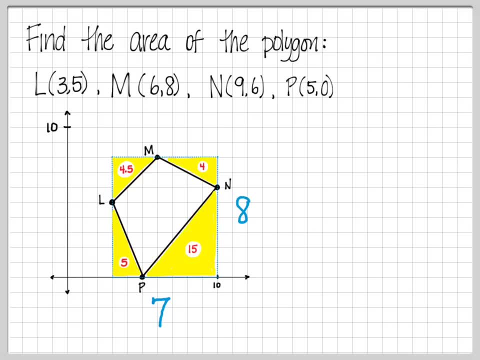 And the fourth triangle is 1 half 2 times 5,, which is 1 half of 10,, which is 5.. So to find the area of the irregular polygon, we're going to take the rectangle, the blue rectangle. 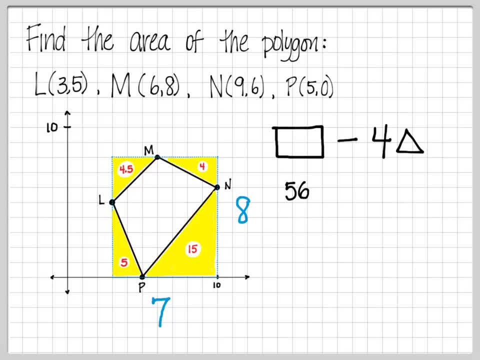 and subtract the four triangles, Well, the rectangle is 8 by 7, so that's 56.. The four triangles: we add all those up and that's 28.5.. 56 minus 28.5 is 27.5..